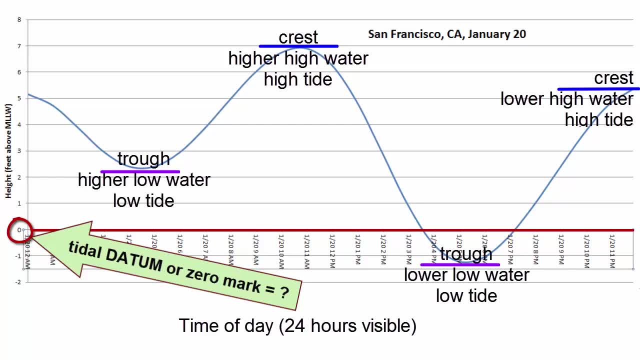 and two low points, troughs or low water or low tide. As the troughs are different in their level, we refer to one as higher low water and the other as lower low water. The zero line on the y-axis is mean lower low water or MLLW. 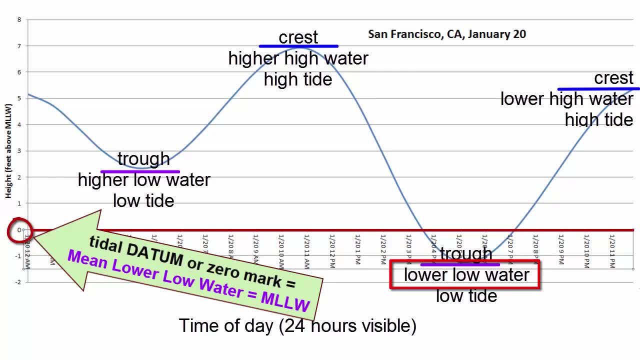 which means the average height of the lower low waters. that happened daily over the past year. So why use this for our zero instead of mean sea level, So that most of our tidal heights are measured as positive numbers and we get negative heights only when the lower low waters are lower than average? 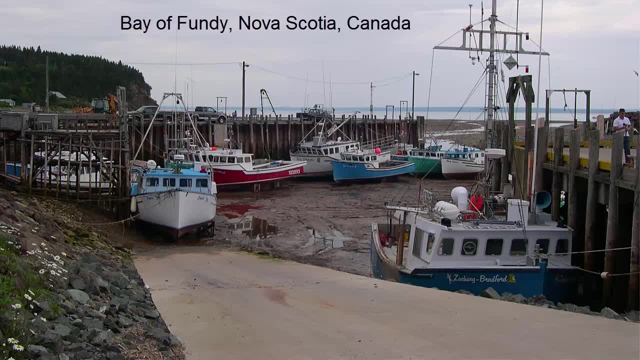 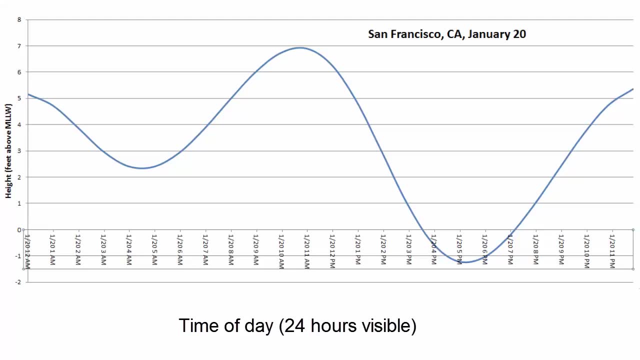 And these are considered special tides, during which much of the coastline is exposed and it's a good time to explore tide pools, dig for clams or clean the bottom of your boat. Let's continue to apply wave terminology from the waves tutorial to the particulars of a tidal wave. 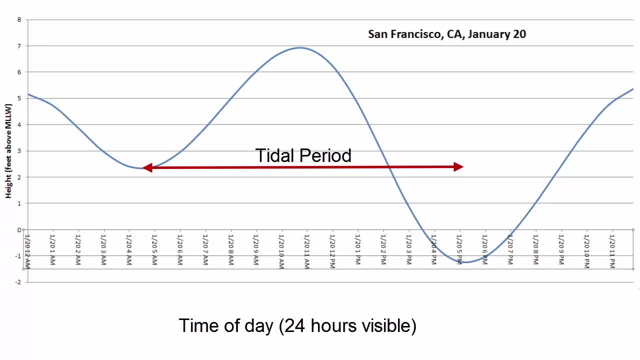 Remember that the period of a wave is the period of a tidal wave. Remember that the period of a wave is the period of a tidal wave. The period of a tidal wave is the time it takes for one complete wavelength to move past a point. 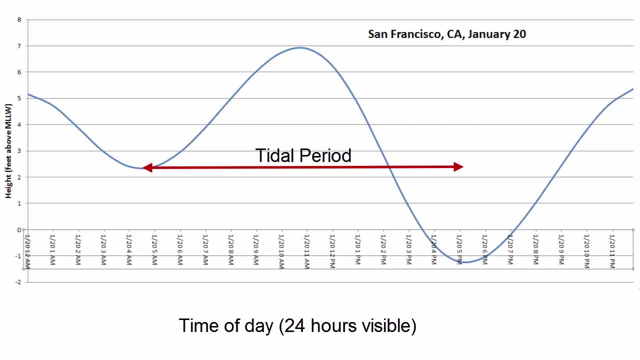 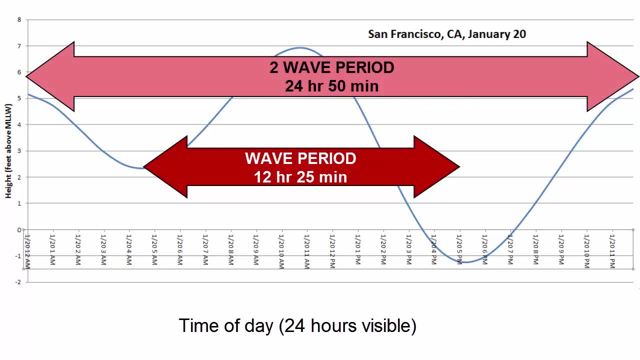 and wavelength is the distance from crest to crest or trough to trough. So the period of one tidal wave is about 12 hours and 25 minutes. Two complete waves, crest to crest and back to crest, again occur every 24 hours and 50 minutes. 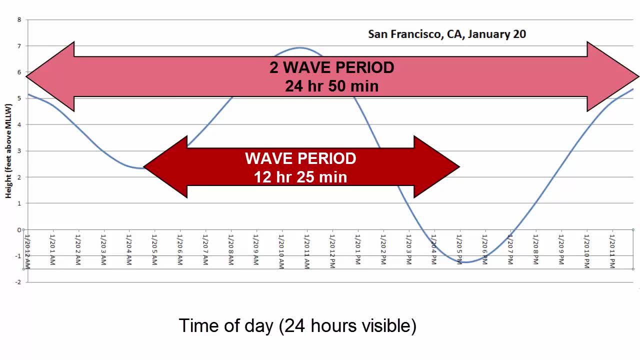 What that means is that if you experience high tide on a beach at 3 pm this afternoon, the next high tide would be at 325 am tomorrow morning, then another at 350 pm tomorrow afternoon, and so on. 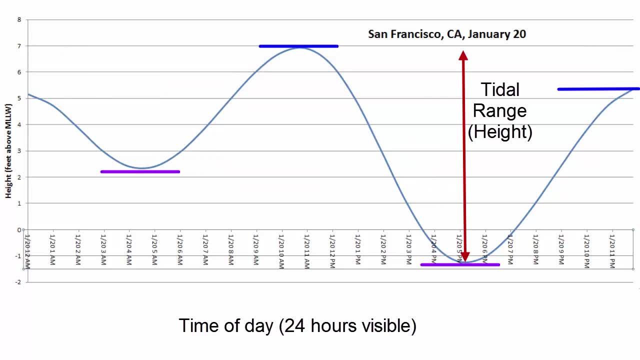 The height of a tidal wave gets its own term: tidal range. The tidal range is calculated by taking the vertical distance between the crest and the trough. When crest or trough height varies, calculate tidal range as the maximum vertical distance from the highest crest to the lowest trough. 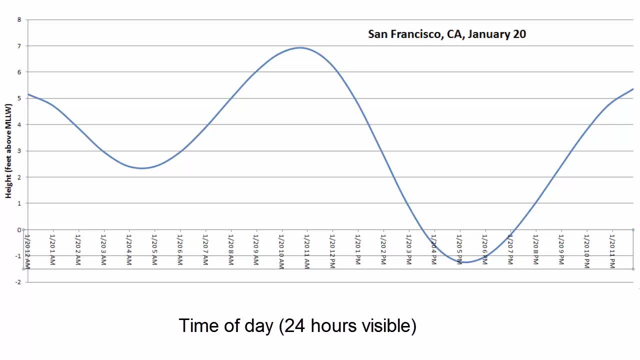 If you were on the San Francisco coastline on January 20th and experiencing these tides at 430 am, you would be experiencing a low tide during which water would be neither rising nor falling. We call this slack water. After low tide, sea level would rise slowly at first. 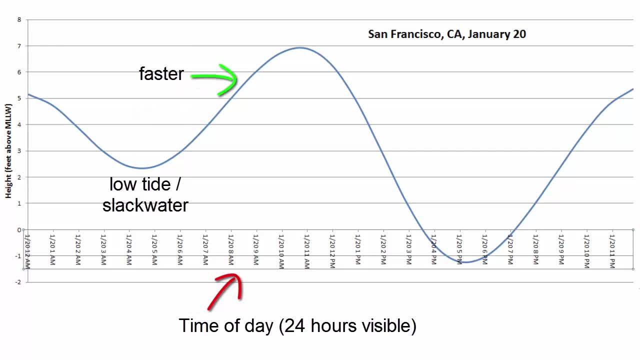 and then faster and faster Water is flooding the land. We call this moving water a flood current. It slows down its advance as 11 am approaches. At 11 am it has reached another still point, or slack water. 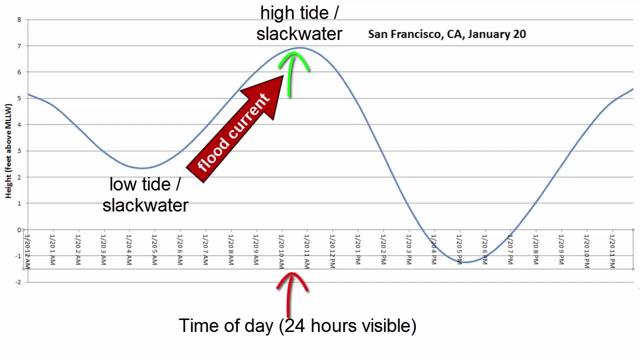 and we are now experiencing high tide After high tide. the water starts to retreat from the coastline, slowly at first, then faster and faster as an ebb current. That current slows as 5 pm approaches, when we get yet another slack water and low tide. 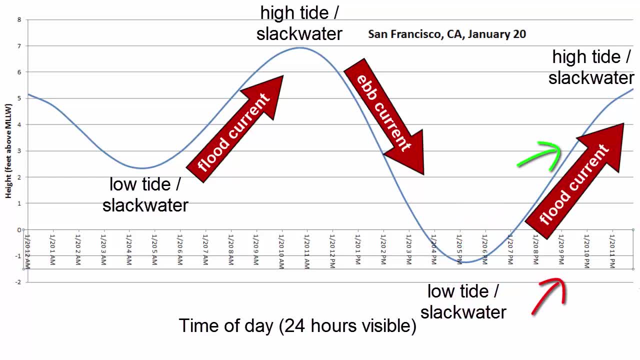 After 5 pm we get another flood current until at about midnight when high tide arrives again, and so on, repeating two waves every 24 hours and 50 minutes. We call this type of tidal pattern in which the land experiences two high tides. 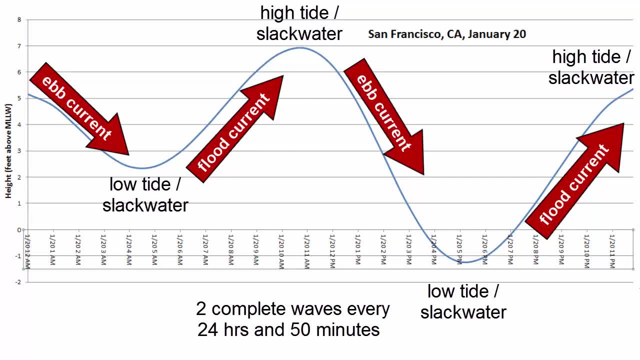 two low tides, two flood currents and two ebb currents in one 24 hour and 50 minute period, a semi-diurnal pattern, Because the water level of the high tides are different, as are the water level of the two lows. 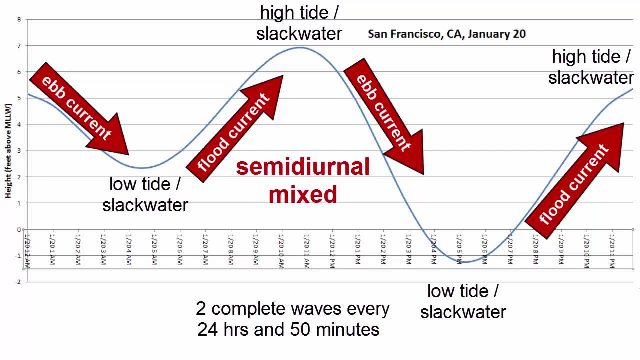 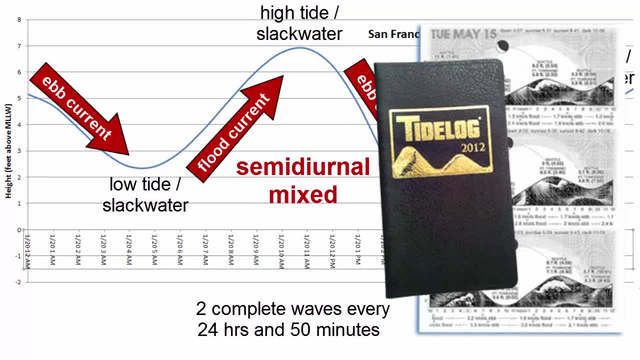 we append the word mixed to the pattern, so it's semi-diurnal. mixed Tides have been studied and data on tidal water levels have been collected for hundreds of years. In fact, their regularity makes them one of the few environmental phenomena. 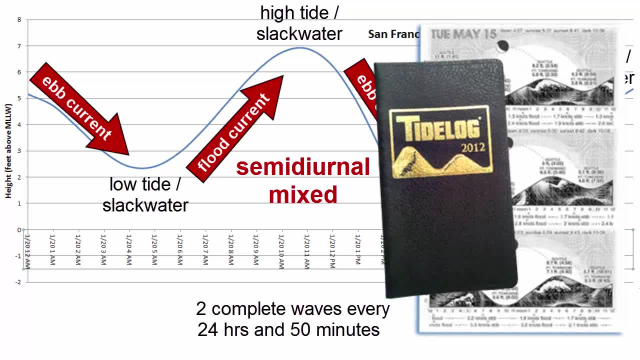 that can be accurately predicted for over a year in advance. Tide books are available with this information at all fishing shops, and tidal data are available freely online If you are planning to spend time along the coast fishing, boating, swimming or picnicking. 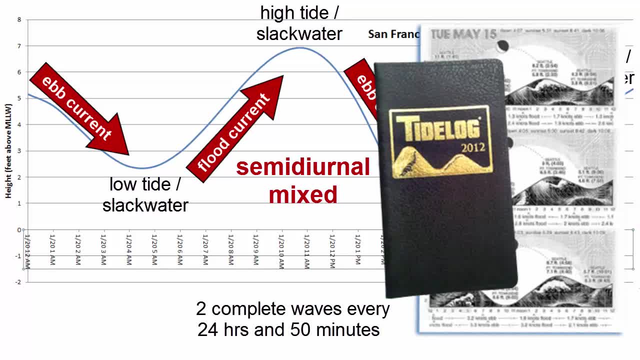 be sure to figure out first what the tides will be doing in your area on that day. While we can predict tidal water levels, tides do not happen at the same time or the same way everywhere. In fact, they vary quite a lot. 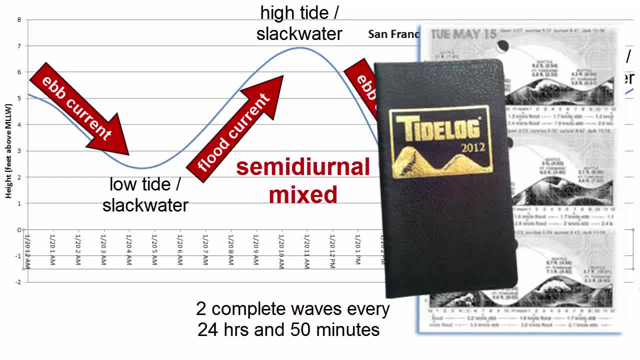 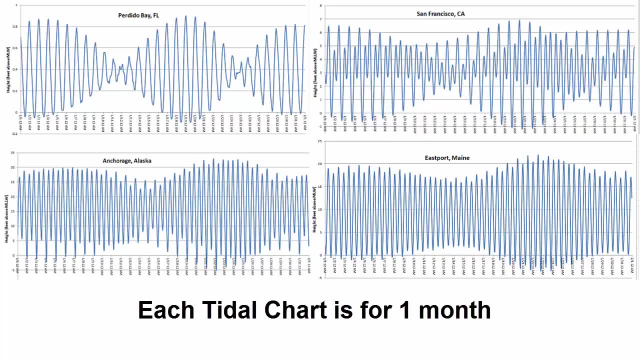 from one part of the coastline to the other, so you must consult the data for a particular beach. Here we see tidal patterns from four different locations across the United States. Let's see what we can learn by studying these data more closely. First, we see that there are represented here. 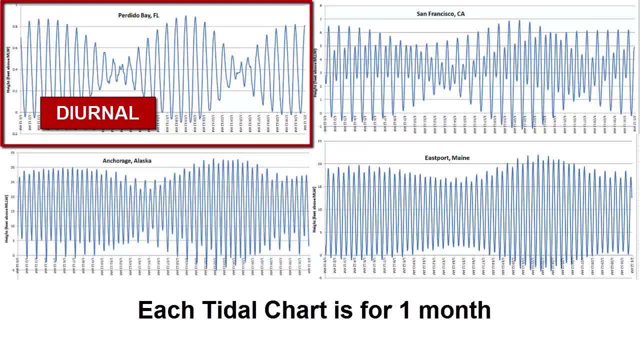 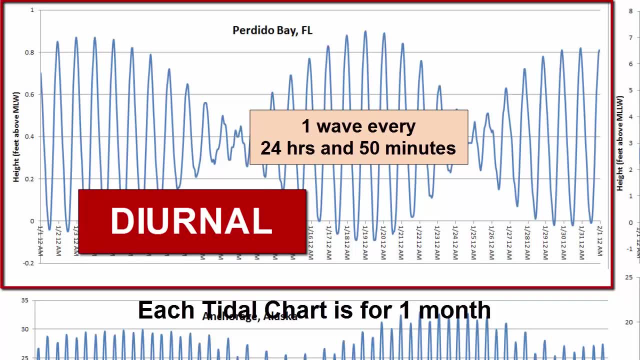 three different tidal patterns. A diurnal tidal pattern means one high tide and one low tide every 24 hours and 50 minutes. This graph shows diurnal tides at a beach in Florida. A semi-diurnal tidal pattern, as already discussed. 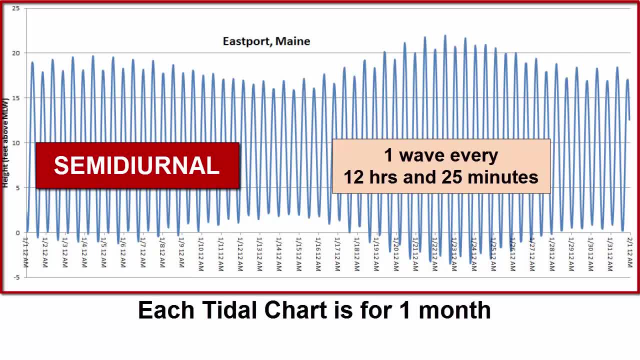 means one high tide and one low tide every 12 hours and 25 minutes, or two high tides and two low tides every 24 hours and 50 minutes. Water levels of each high are roughly the same Water levels of each low. 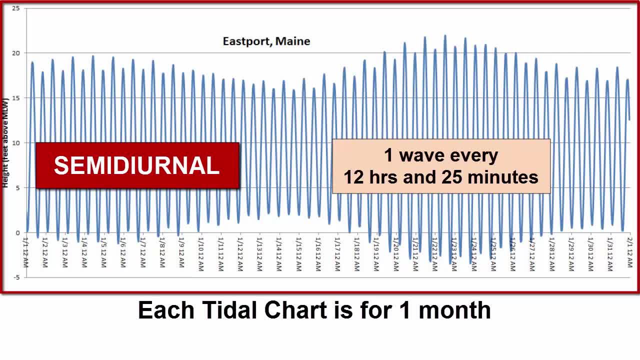 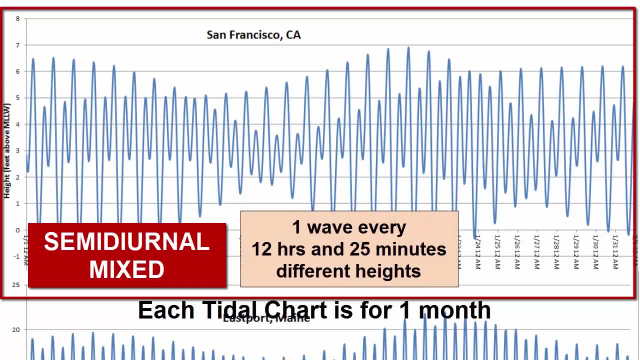 are roughly the same. A semi-diurnal mixed tidal pattern means they behave exactly like semi-diurnal tides in their periodicity, but the water levels of the two highs can be quite different, as can the water levels of the two lows. This semi-diurnal mixed pattern 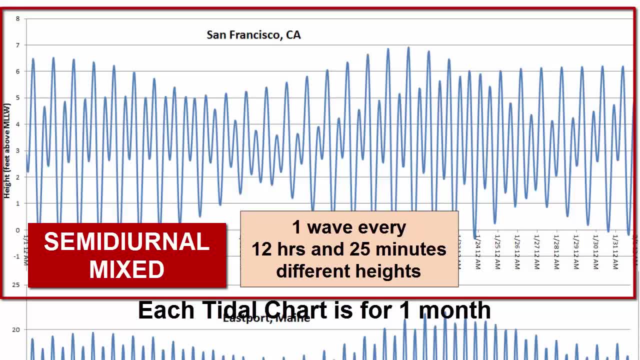 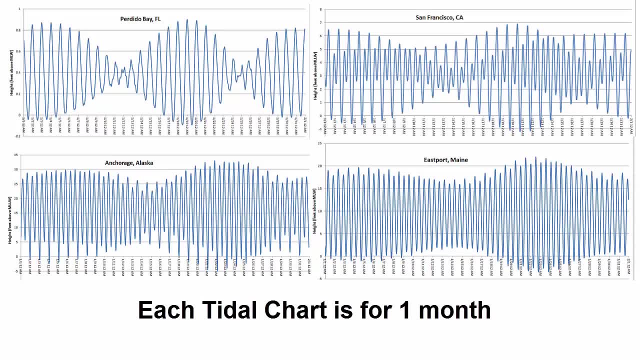 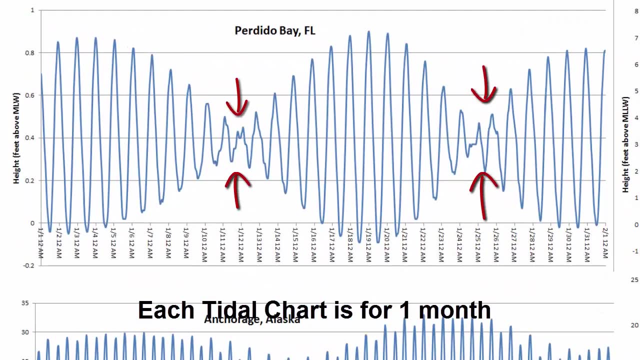 is from San Francisco and similar to what we've already discussed. The other thing we see by studying tidal patterns from different locations is that tidal range fluctuates on a two-week period. Looking just at the tidal chart from Florida, we can see that twice during the month. 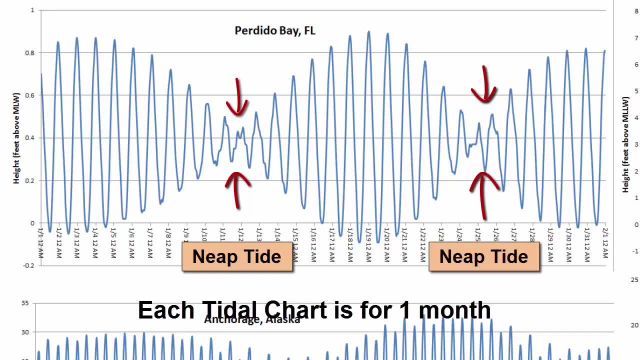 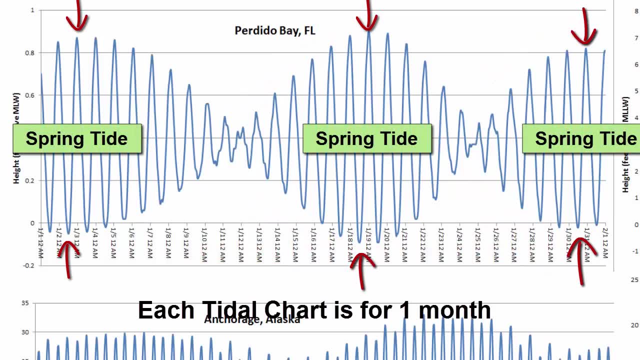 the tidal range becomes much smaller. We call those neap tides. After each neap tide passes, tidal range grows again until it reaches a maximum tidal range, which we call spring tides. After spring tides pass, tidal range again diminishes. 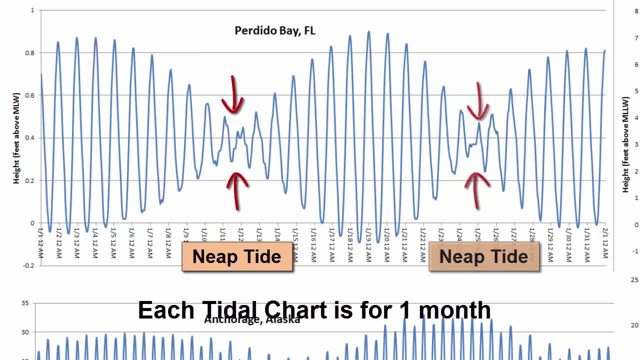 for another week until it reaches another neap tide. And it continues this way every week, moving from neap to spring, then back to neap and back to spring. Spring tides happen every two weeks. Neap tides happen every two weeks. 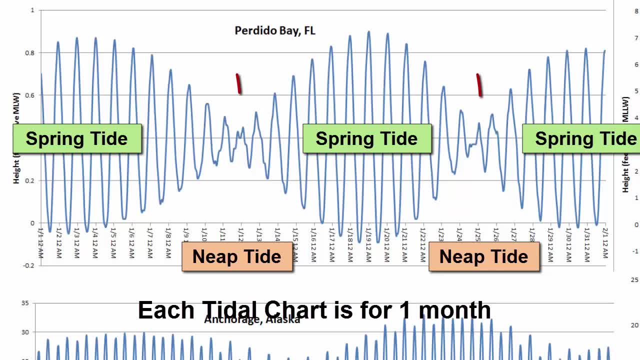 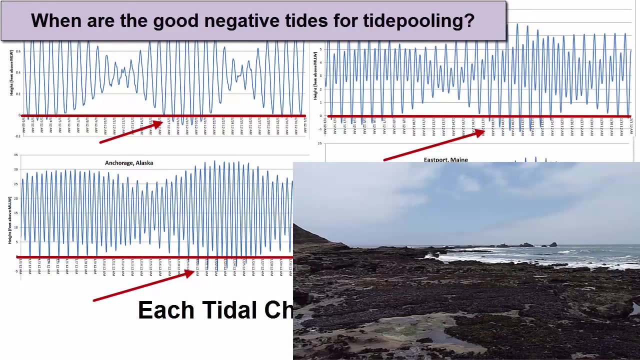 Notice that during neap tides we get both the lowest highs and the highest lows. The opposite is true for spring tides, which have the highest highs and the lowest lows. At which time would you expect to get the negative tides that indicate really low water? 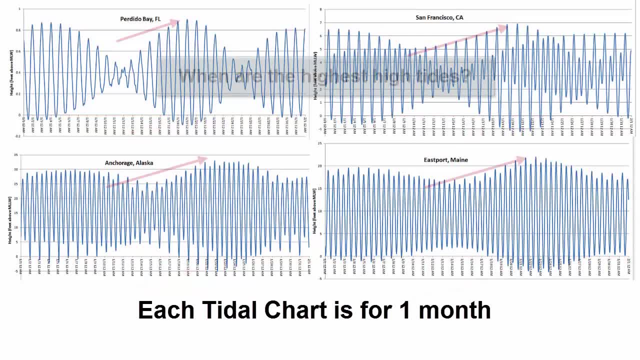 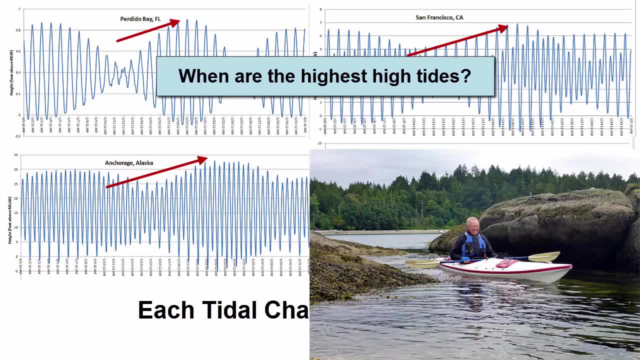 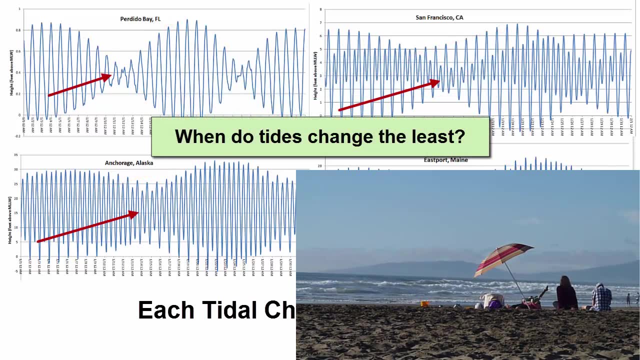 and good tide: pooling The spring tides. At which time would you expect water levels to be highest through normally shallow waterways? Spring tides- At which time would you want to plan a beach picnic so you could minimize water level changes around your picnic site? 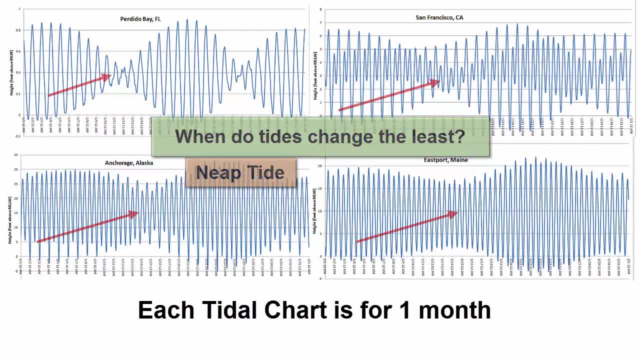 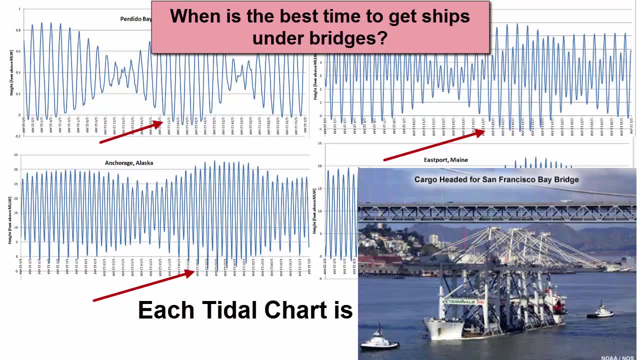 Neap tides. Finally, there are some ships that must time their entry to San Francisco Bay to make it easier for them to pass below the Golden Gate Bridge without hitting it. They are looking for the lowest water levels. When would that be?